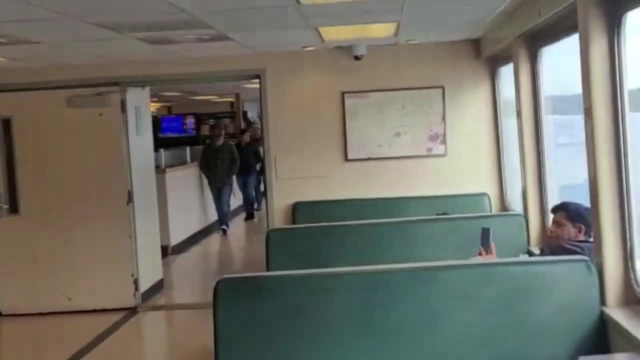 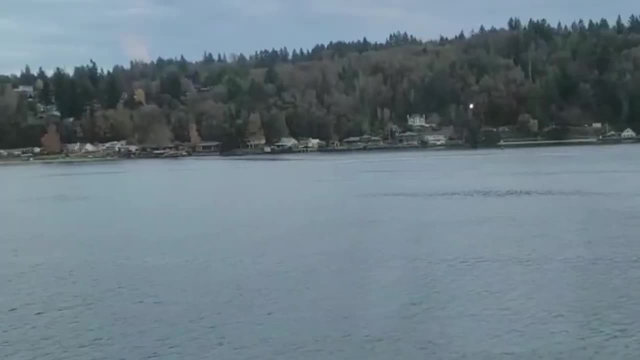 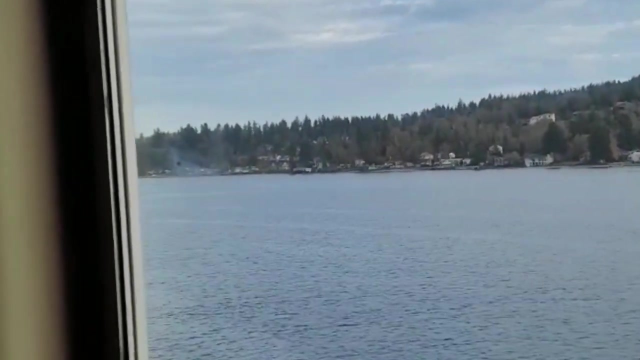 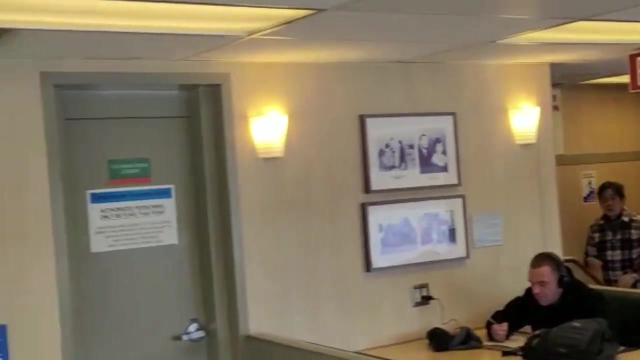 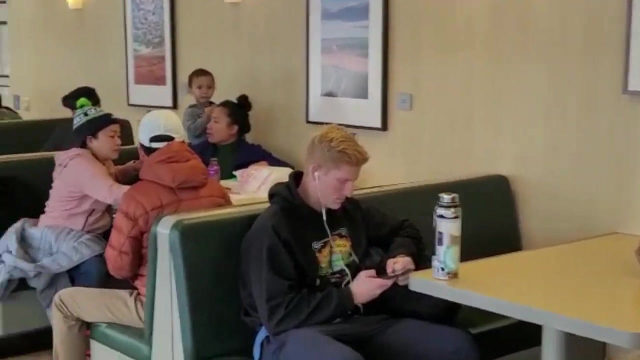 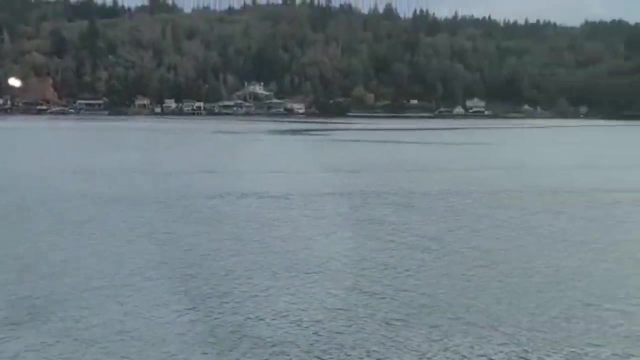 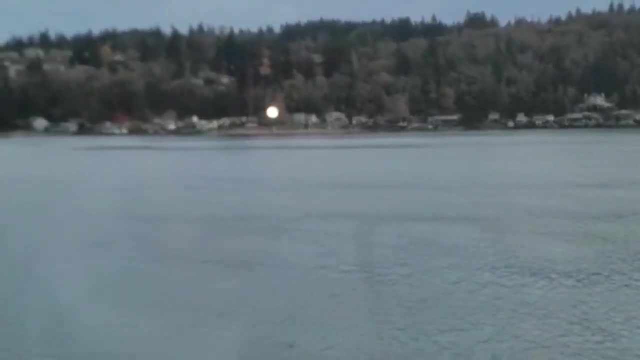 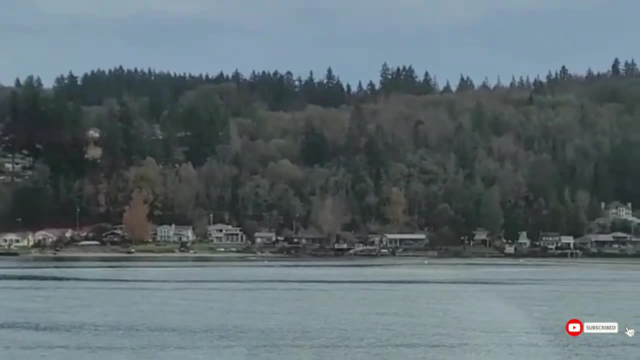 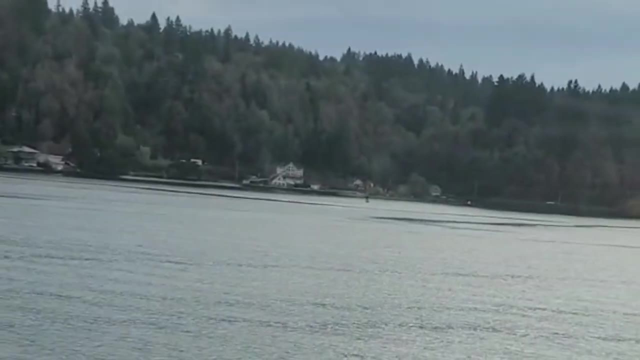 Yeah, yeah, Look, I'm in line with the stars. I'ma sink with the earth Ten toes deep, fly with child from the turf. I never switch sides, like even when I die. I'ma ride for the squad. lot of ties in the hearse. 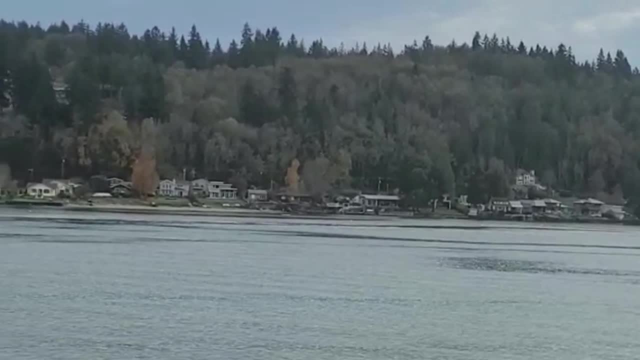 I've been on the vibe kinda hard to describe. I'm in between, I'm good and it's fine, but I'm tired of the grind. Then I come alive in the night to realize I'm in the middle of the time of my life. I'm never so packed for the stack, never lied on the back, Got a bag from the way that I write it, queen, looking Tyson Through that. I survived doing 80 to the house. Then I hit it to the sky, changed gators on the deck. 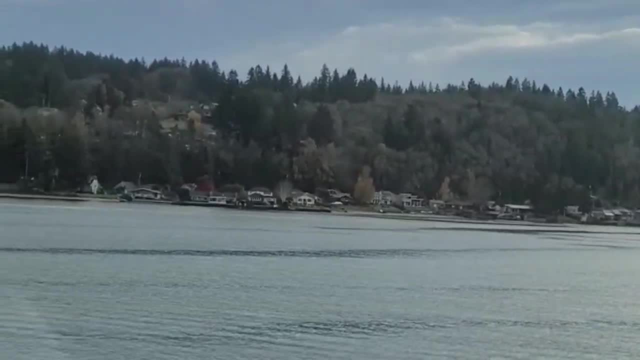 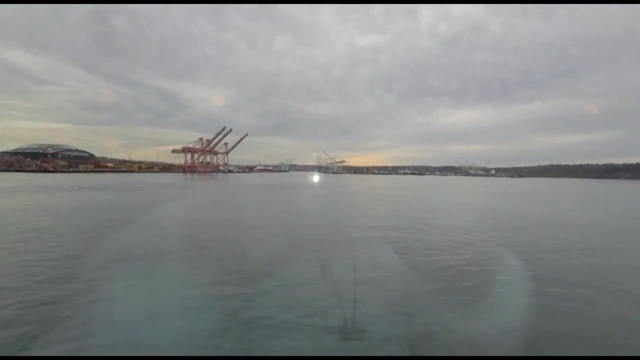 Tyrant, talking to the grip and the face. be still Like I hit stuff fade. we all with the same. We all want a meal in the safe. I wanna live Like I'm trying to get your light man Trail spill from my lips, feel bent from the bit. 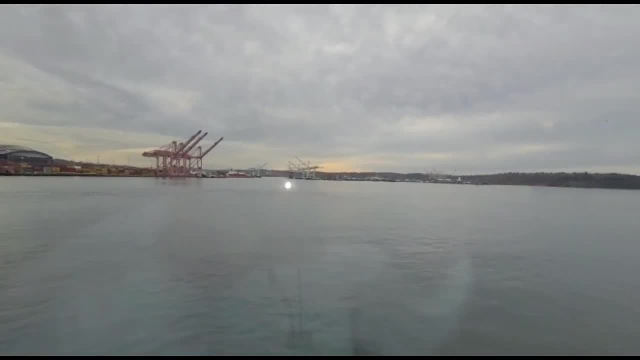 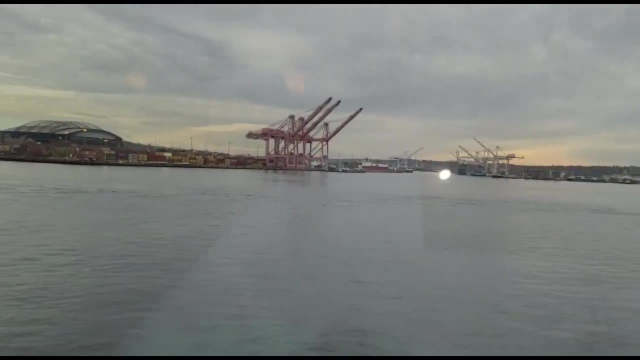 Take a sip till I pass out, Try and get grip, but it don't make sense, Cause you could lose life on this fast route. Yeah, turn thoughts to a cash cow. I might flip that to the glass house. I don't need the accolades. I'm in love with the chase. 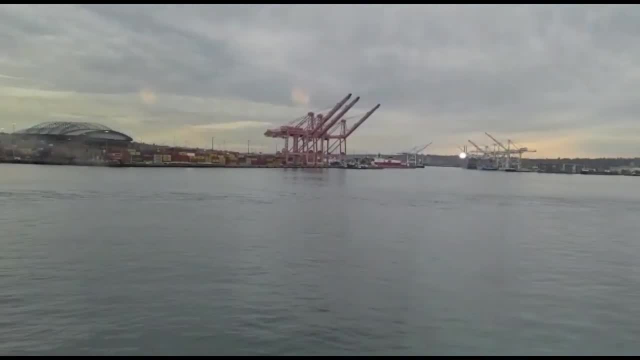 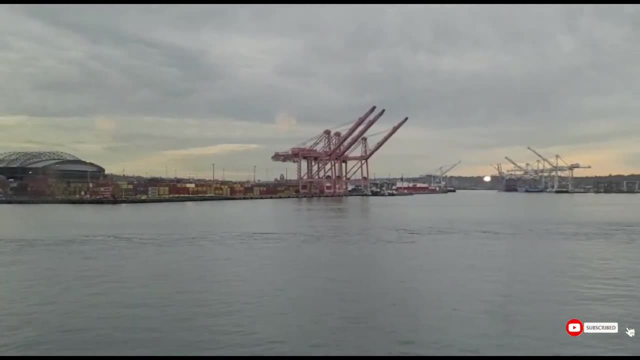 I just wanna eat. save a spot at the table. Beats with the slack pin myself on the map. You long with the wind, but we, knowing that it's capped, Five hour flights couple nights at the flat, To be real, couldn't see me making moves while I'm at. 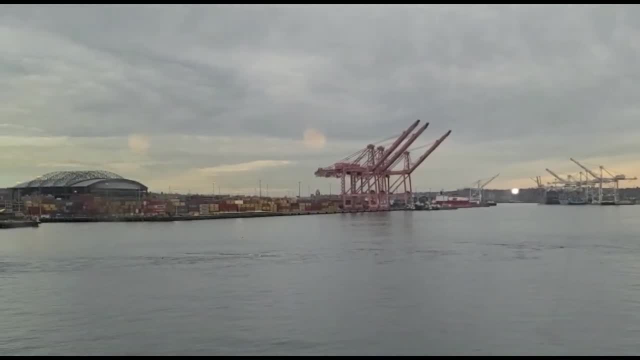 I'm still on the grind living time. when I chat I'm burning down sage, keep the demons away. When I write it, give a piece of myself to the page. I don't do it for the praise. love, that's just how I'm made. 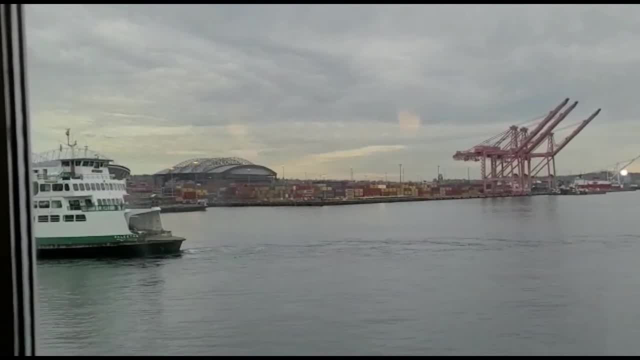 See the truth in the glass, in the mirror. Do it at me, old man, trying to pass in the fear. You're the first one to talk, but the last one to hear. Eyes blurry, but I couldn't see that And he cleared them. 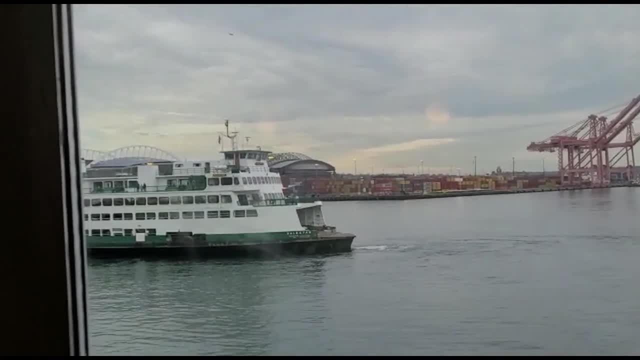 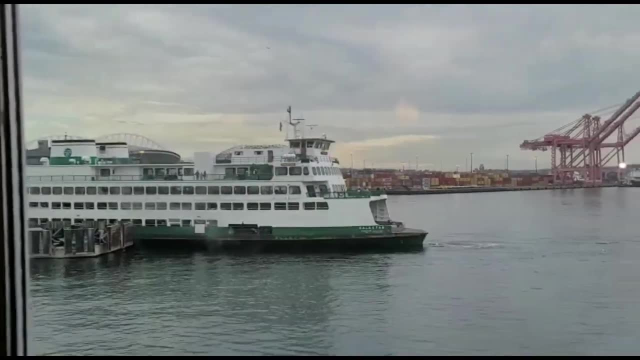 Start to feel like I'm on one. Settle in. I'll be here for the long run. I'm a slave. for the cash got snakes in the grass, No brakes on the ad, but it's all fun We done. seen it all, heard it all. 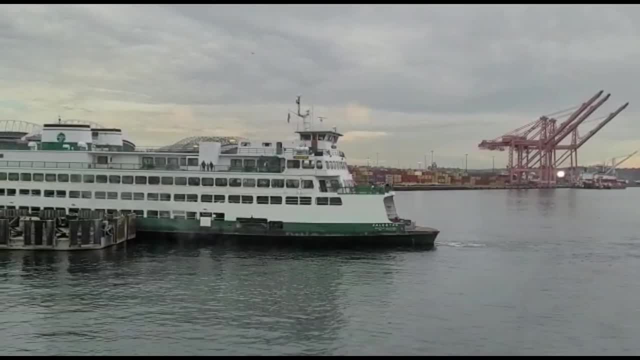 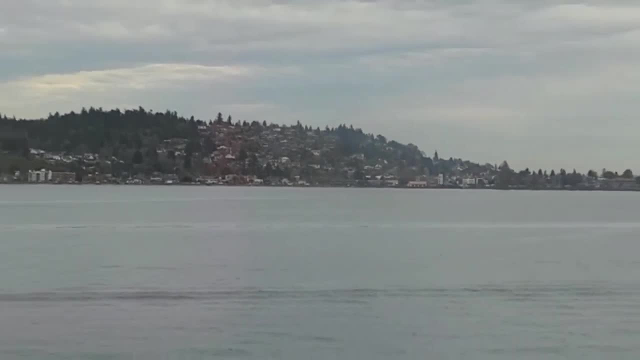 Heard enough, give me space before I murder y'all. Ten bad b**** there. I'ma curb them all. Twelve missed calls and I still made a curtain call Here to light it up. lighten up, Hear them talking. they ain't right enough. 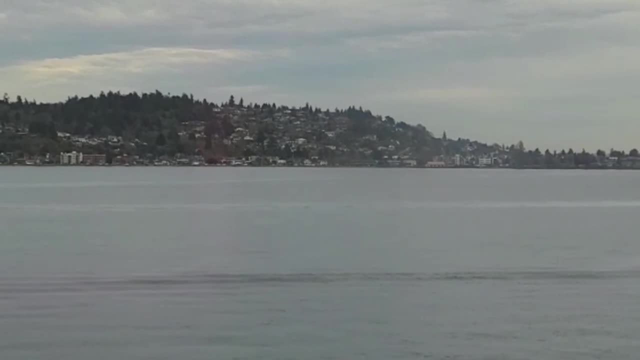 Tighten up everything that I came for I left with. I don't bang sets, I just bang on the set list. Don't pass up. but when I came for the breakfast, Put me in your prayers. I might put you on a guest list. 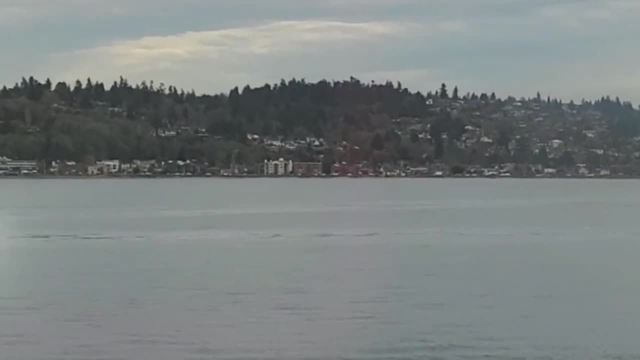 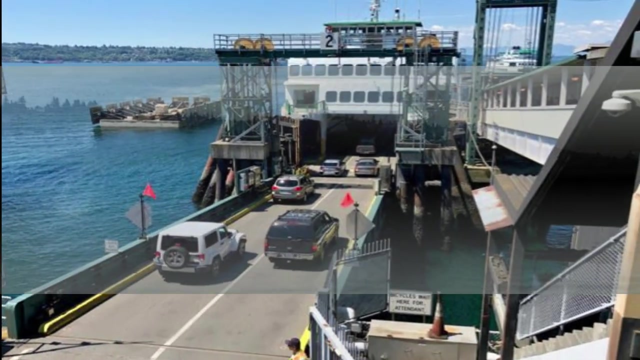 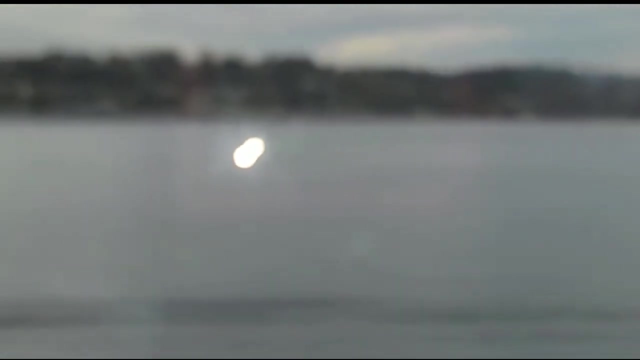 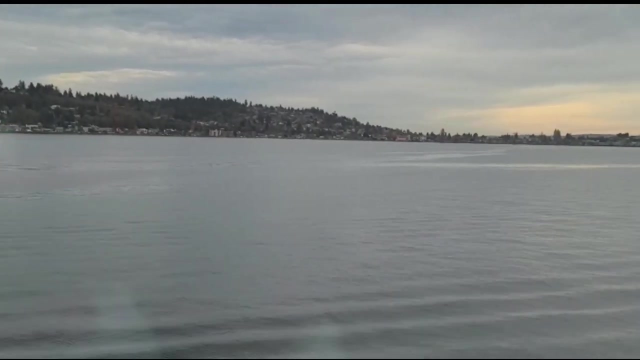 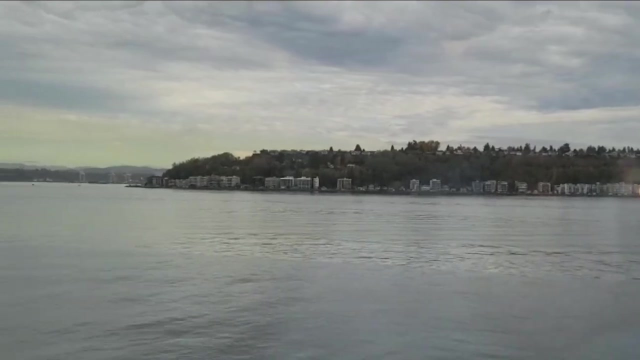 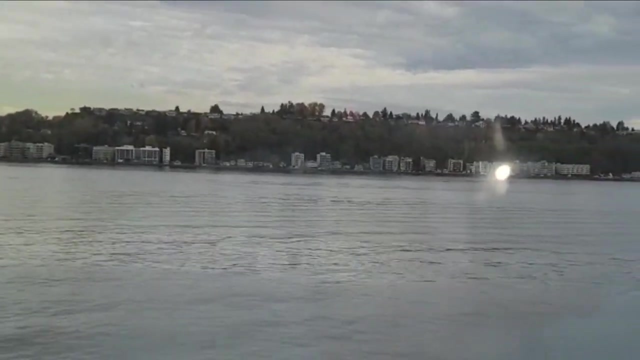 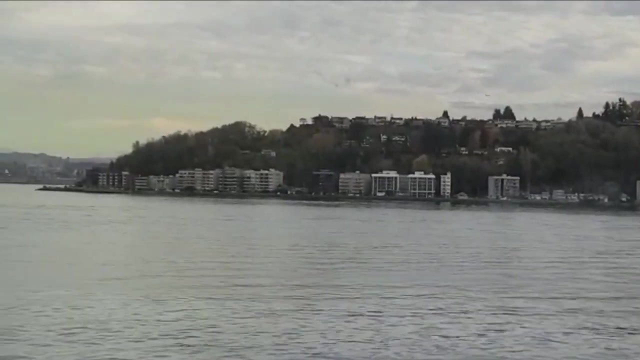 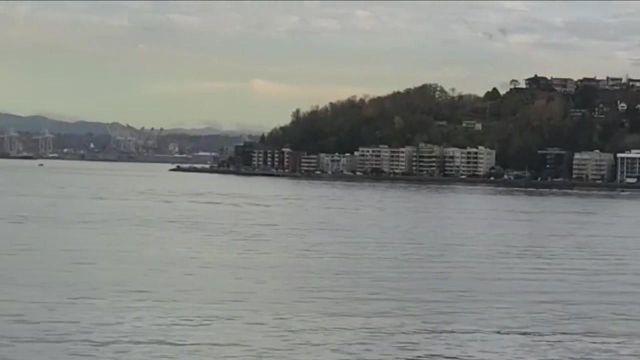 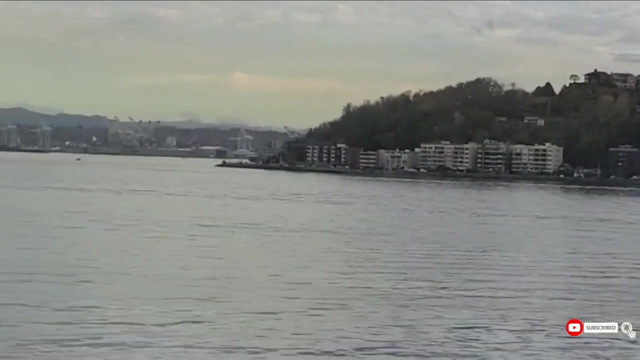 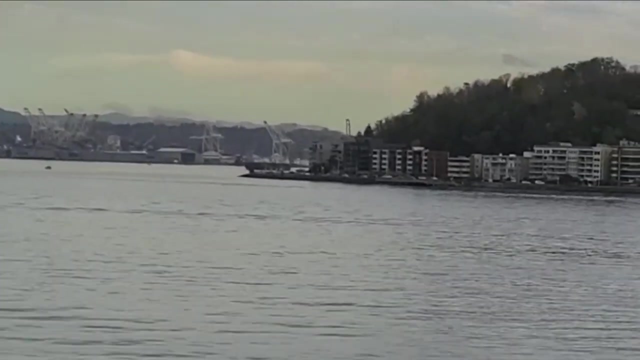 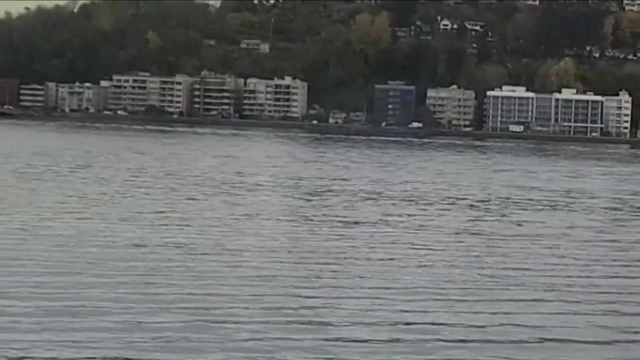 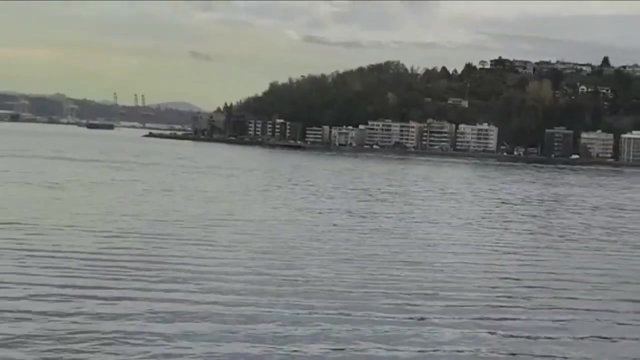 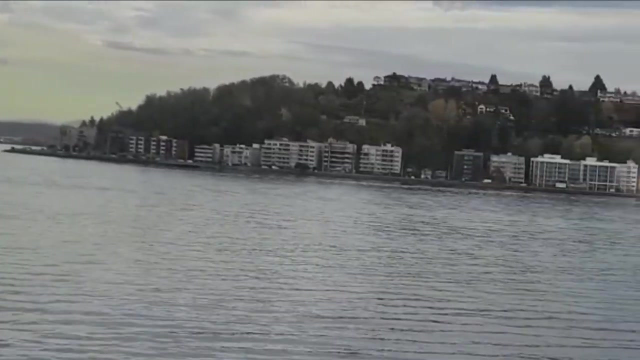 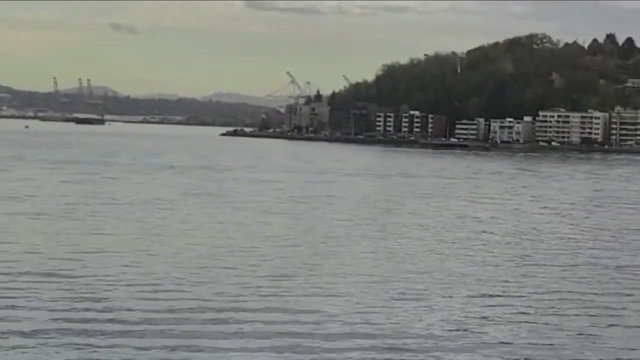 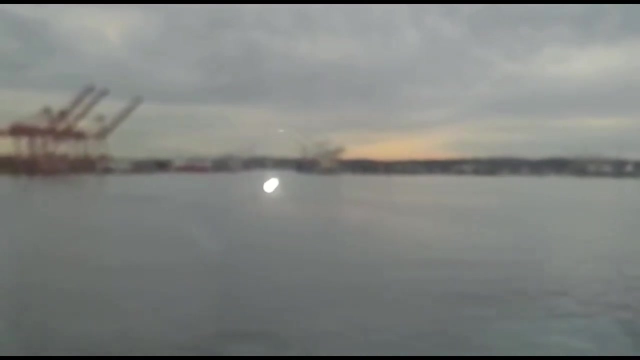 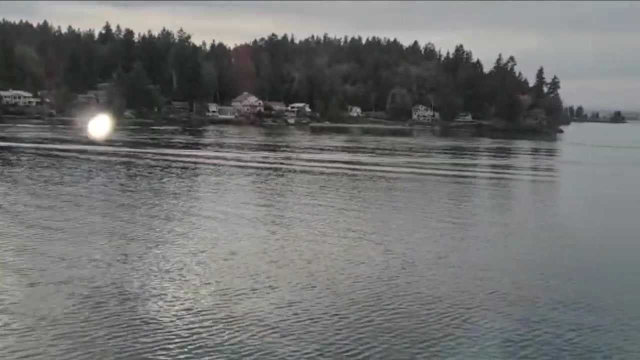 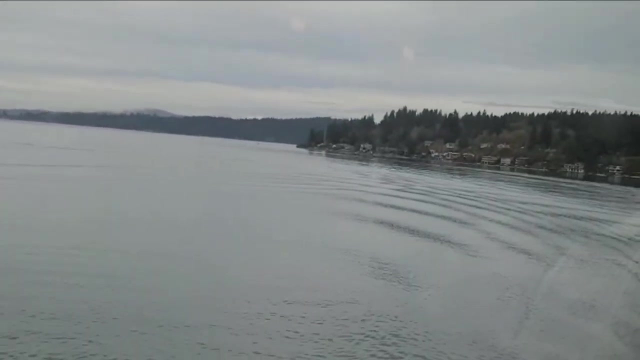 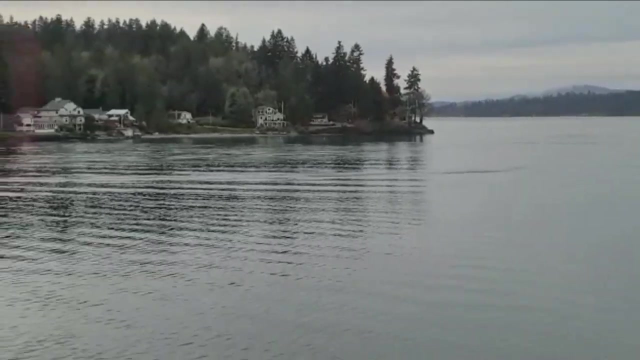